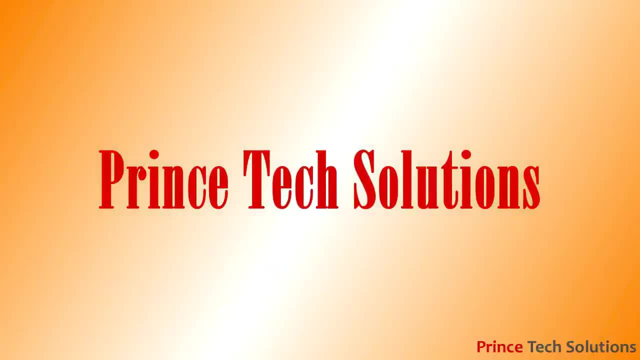 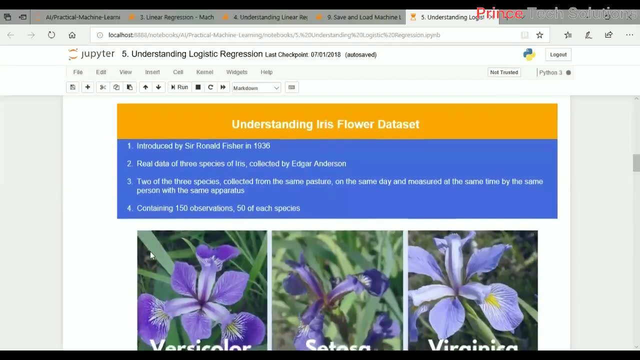 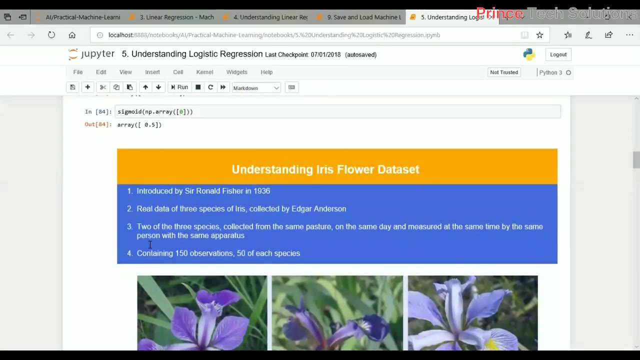 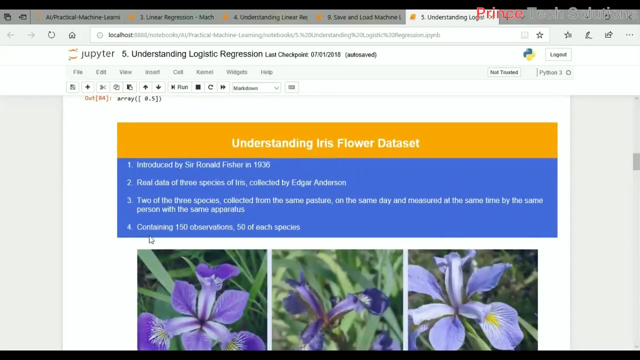 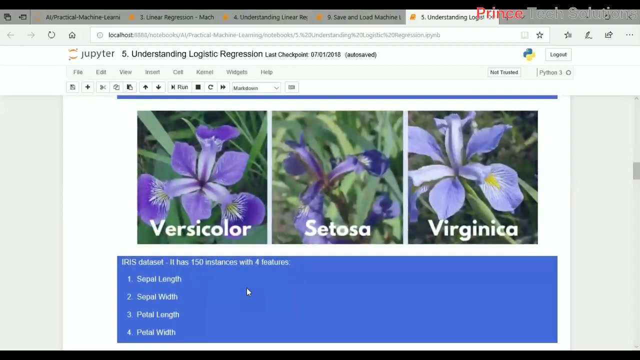 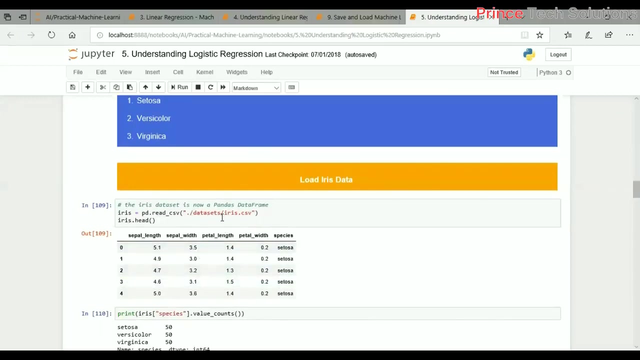 So the data set we are taking is iris flower data set, one of the famous data set. So this here, with the help of logistic regression, we will classify it into. so in regression, obviously you know that classification- last one, It's just numbers And here the target is nothing but classes. Okay, Yes, yes, So I'll just quickly give you the brief about the data. So this is what the data so I'm I'm using here CSV. This is what the external CSV loaded into this iris. So iris is my data frame. Okay, So this is. these are the four different features for this data. Yeah, 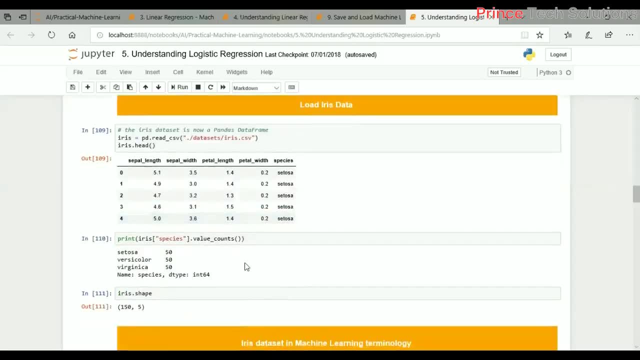 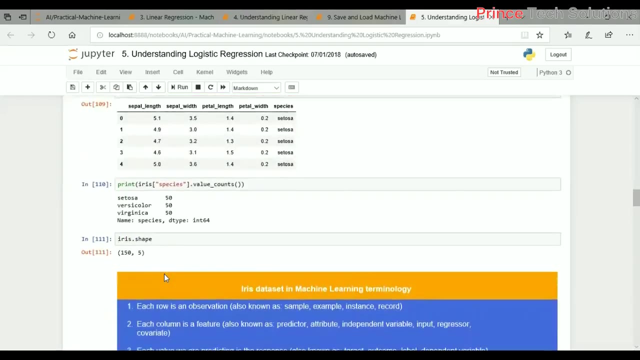 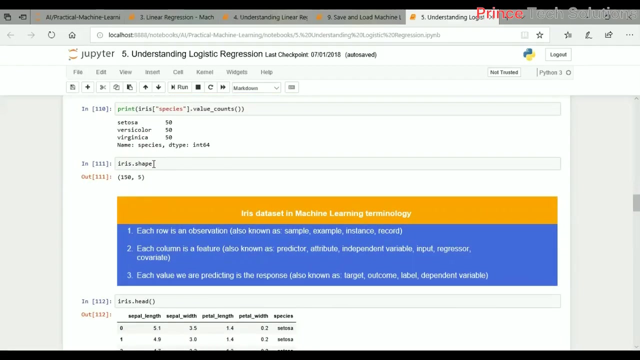 Okay, And these are the classes. Okay, I can get the classes of a particular values, like spaces, like this classes. We say that set us off 50, versicular 50.. These are the samples for each. Okay, Then iris dot shape, we can check using shape function property. So 150 by five, So there are five columns and 150 rows. Okay, 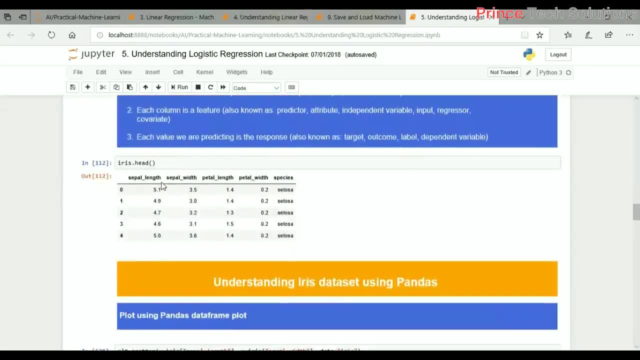 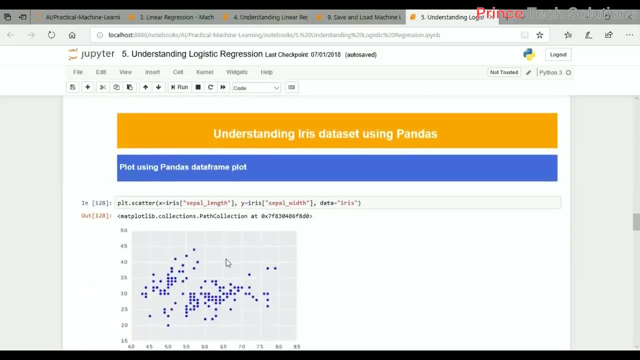 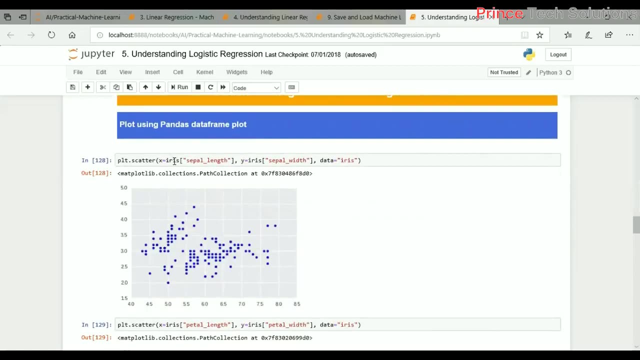 Okay, Now we'll just do a scatterplot on one of the Parameter or feature. So from the x axis will, from the x, we will say simple length and here simple beat, from the data iris. So this plot look like: what is? what is data equal to iris? So from the x axis we'll say sepal length and here sepal width, from the data iris. So this plot look like: what is? what is data equivalent iris? No, No, No, No, I'm not sure of that. 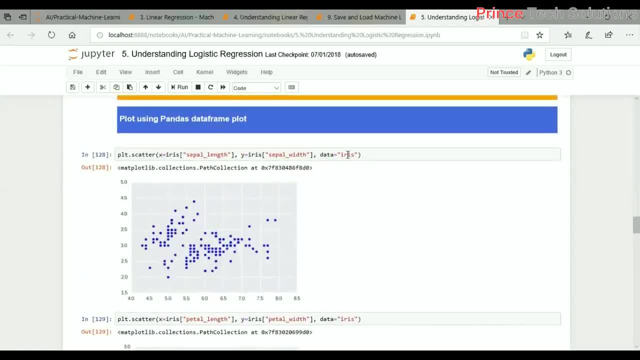 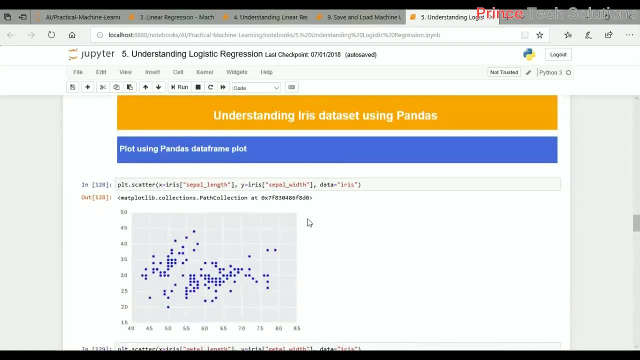 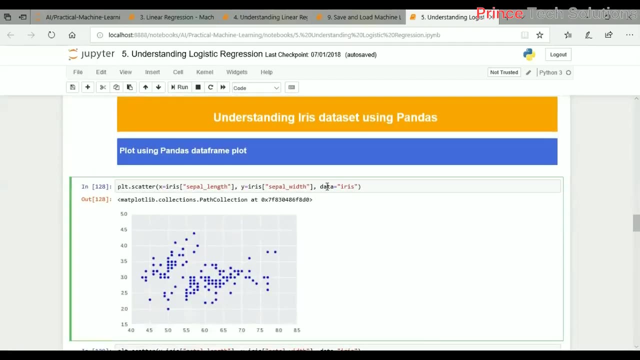 Yes, but is it? Yes, Yes, Yes, Yes, Yes, iris is nothing but my data set. this, but okay, okay, but can write unit as a string, is it? yeah, it's a what you can see, because only to know where, from which data set you want, okay, okay. 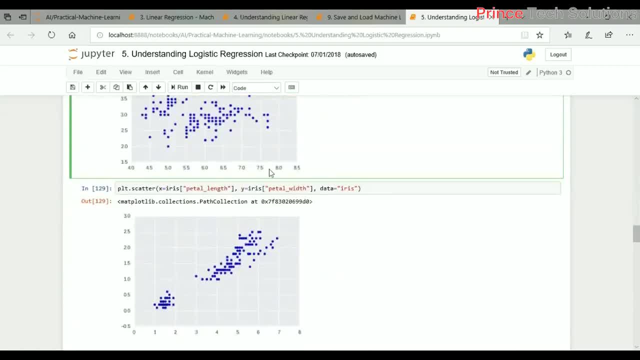 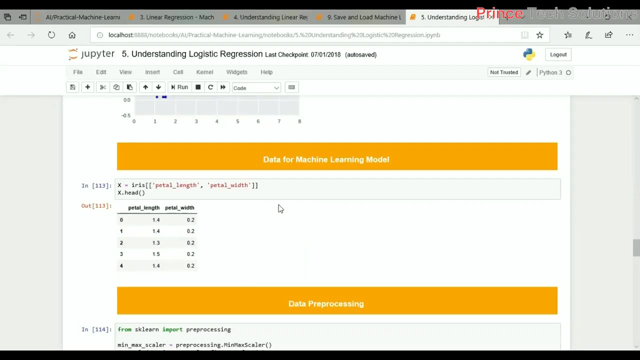 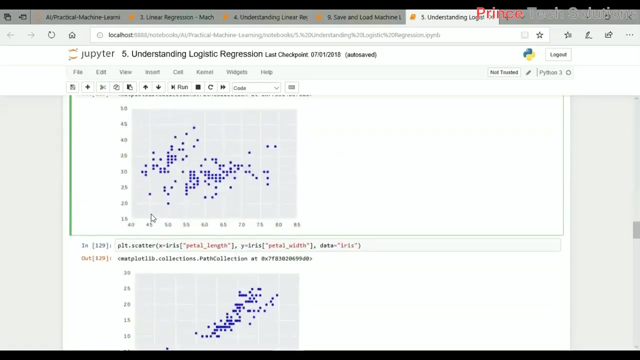 and using petal length and petal width. so here you can say that: how much of fatal? yeah, now here for classification. we will take only two features. so petal length versus fatal width. okay, and because if you observe this, this plot gives you more classification. consider and. 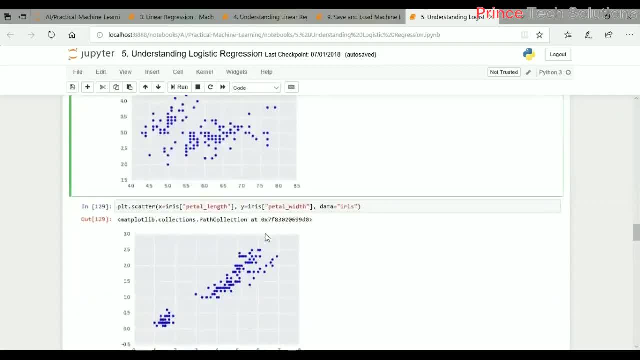 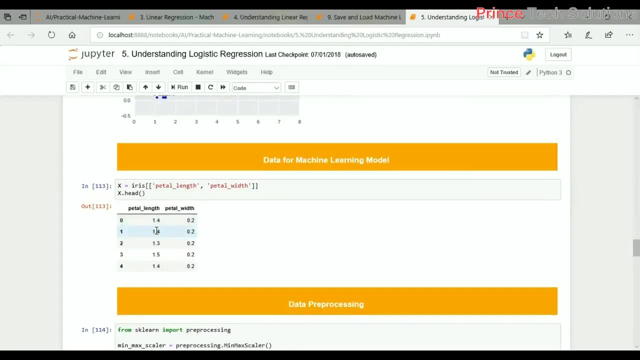 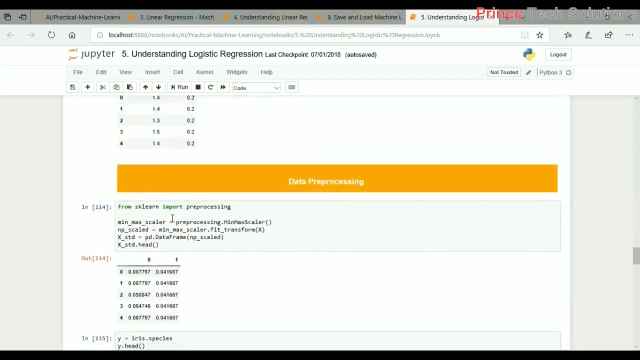 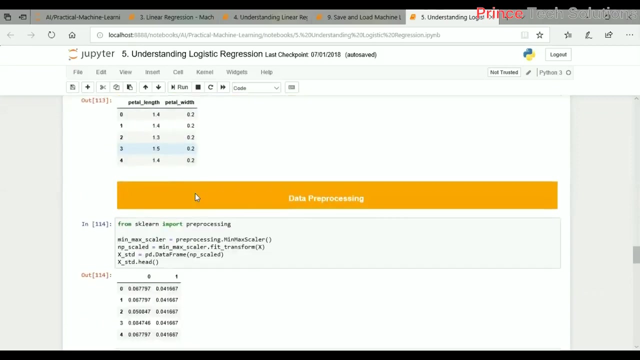 consider and consider, because if you observe this, this plot gives you more. yes, yes, if you observe difference between these two. okay, correct, we'll just correctly take this petal length and petal width, so this become xr and we will just do some pre-processing because these values are not in the same range. okay, so we will use this min max scalar thing. 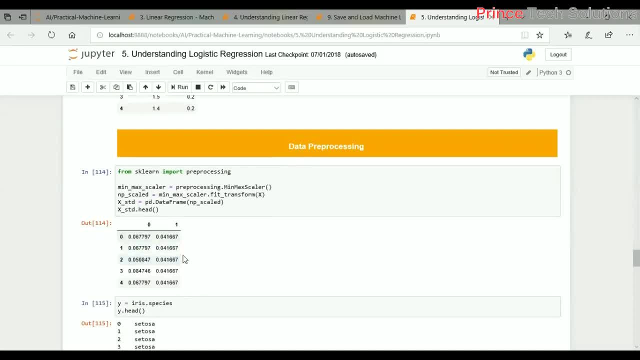 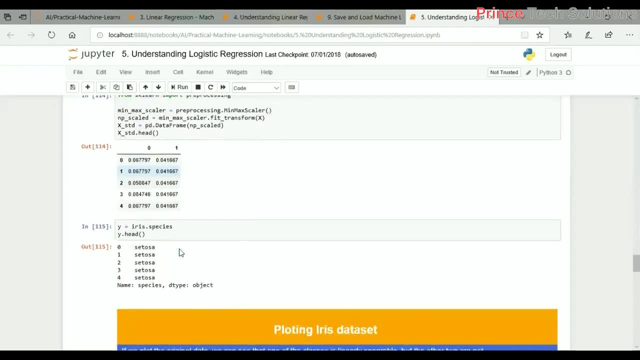 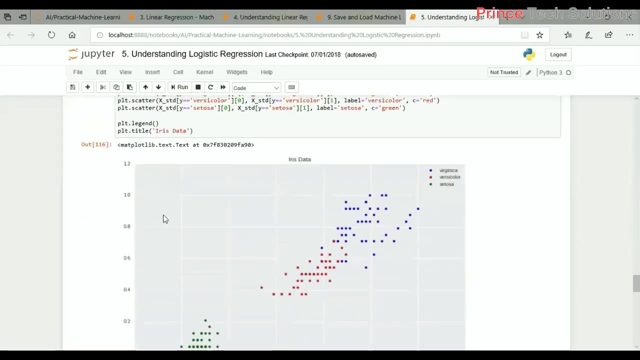 to put the all the values into the zeros and one. so this, this functionality, pre-processing- helps you to put the things in in a one range. okay, and this is what our y. now we will plot based on the different things. so this plot gives you the clear idea: where is the virginica? where is versicolor? 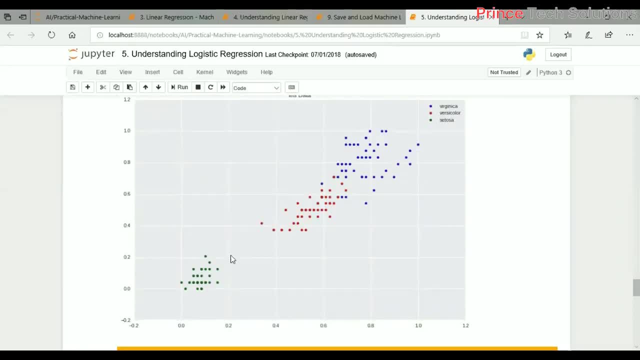 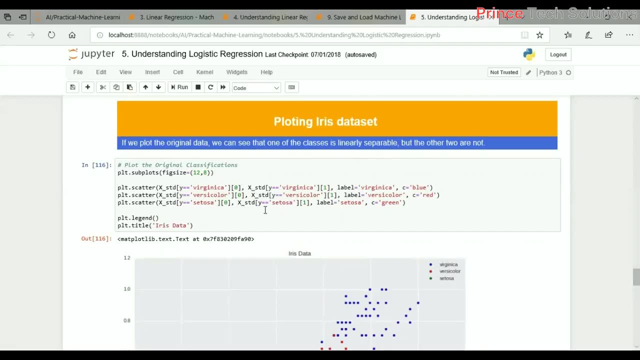 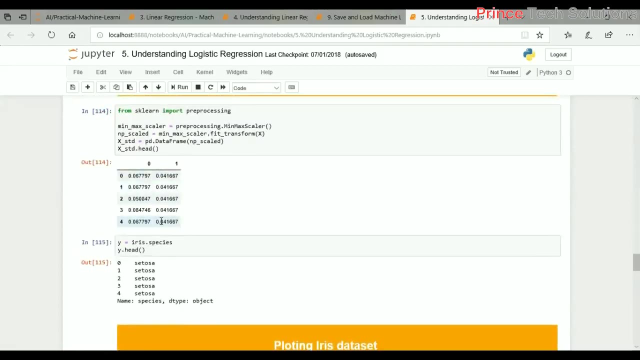 and where is the set to something so you can see that this is what the separation is. okay, yes, yes, so i'm just trying to figure out using some values. so so if before, if we, if we plot before this, uh, pre-processing it not look like this, maybe, maybe these are not in a one range. 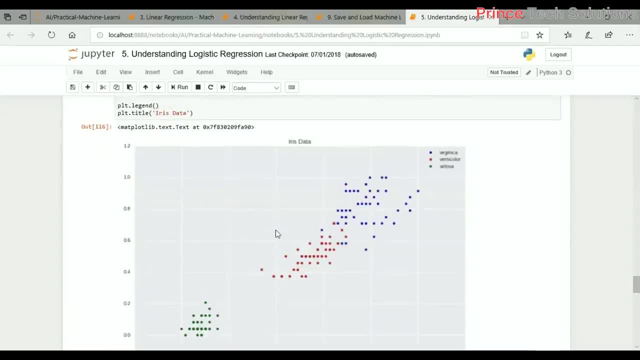 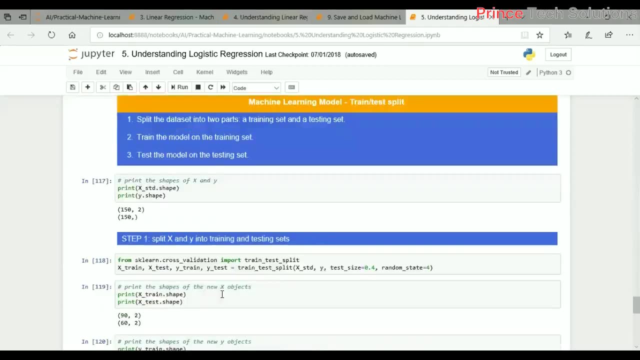 okay, so that's the reason. we just pre-process this data and we put it into zero and one. okay, yeah, now these are the simple things. we, uh, we just split the data into thousandideo twenty percent. so at this point, uh, when it ends, we enter the arbitrary. 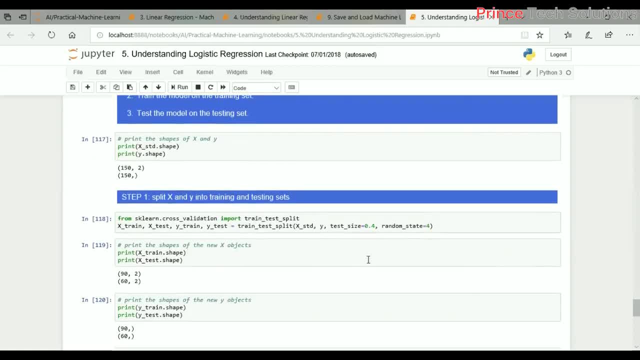 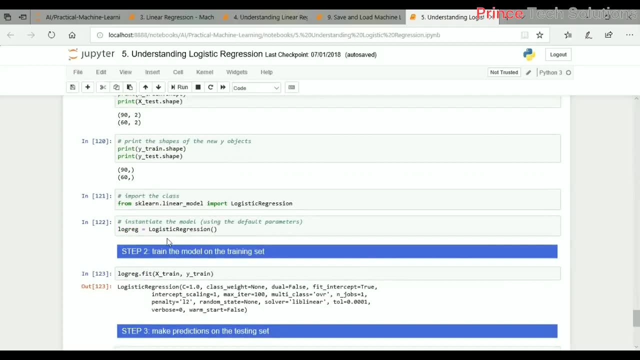 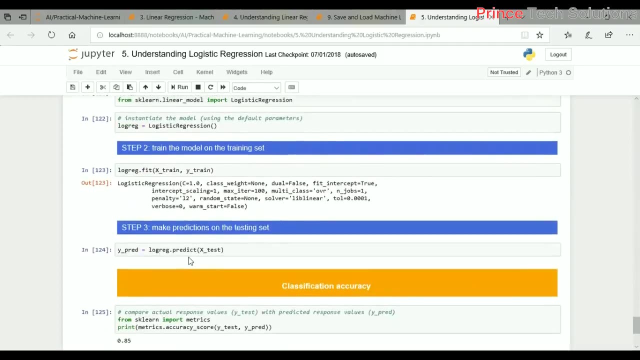 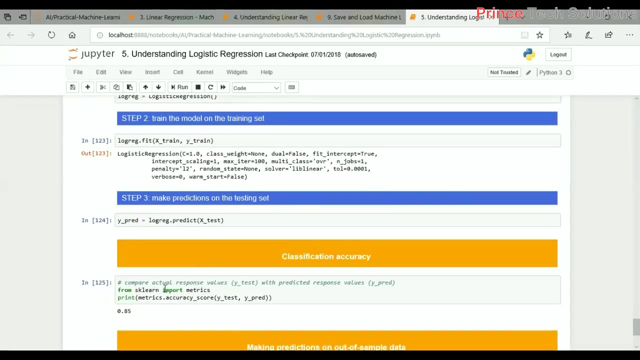 breathing function. Normally those two that we set from zero to infinity will be the same thing. i mean, you observed that, for example. Okay, for example, in our government creation, we created two-part train and test. By keeping this test sizes forty percent and we choose this logistic regression. we created the object, we fitted the data over the training, we predicted using